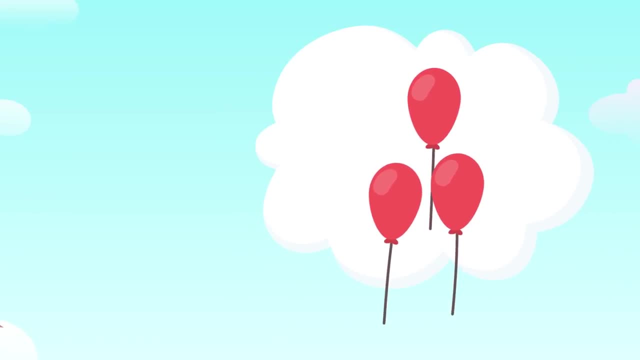 Would you like to practice for a while? Let's find out how good my aim is. There are one, two and three balloons, and I'm going to see if I can burst one of them. The subtraction we need to do is three minus one. 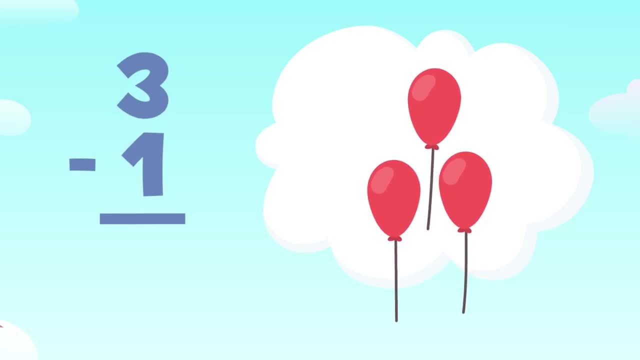 This means there are three balloons and I have to burst one. I'm going to aim well to see how many I'll have left. Ah, here I go. Fantastic, I aimed well, Let's see how many. there are now One and two. 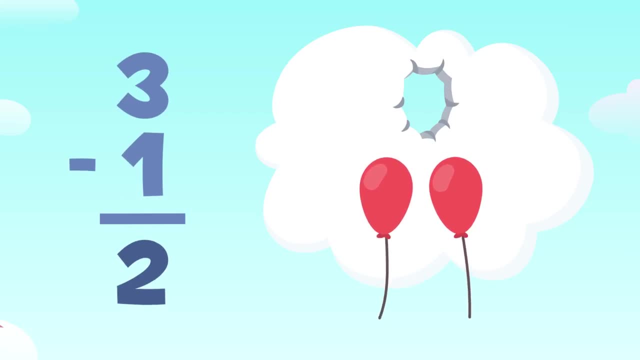 There are two balloons left. The result of subtracting three from one equals two. My aim is truly good. Some balloons are flying away. There are one, two, three and four balloons And I'm going to try to aim correctly. 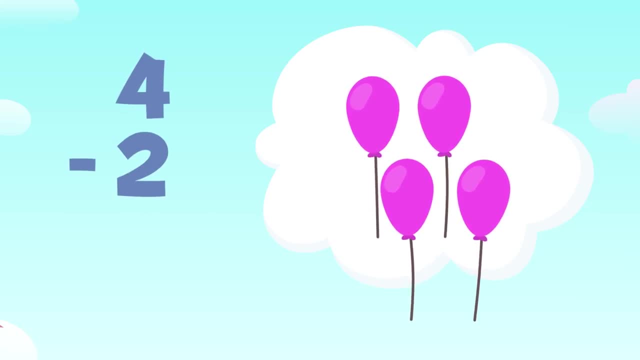 One to aim at two of them. how many balloons will there be left? we need to subtract four minus two. this means that out of four balloons we need to take away two. I'm going to aim well to see how many I'll have left. one and two. yes, let's see how many balloons we've got left. one and two. there are two balloons left. 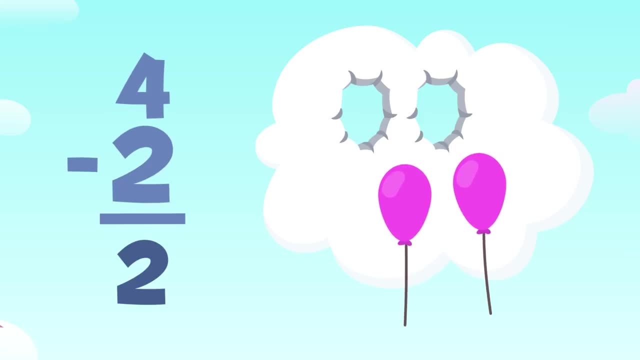 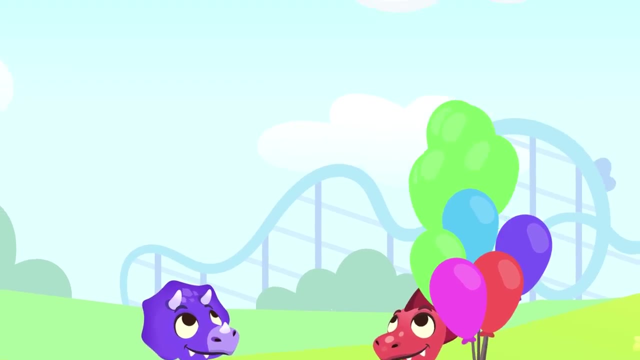 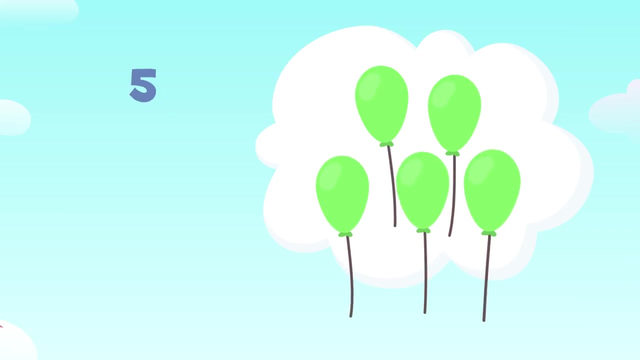 the results of subtracting four from two is two. I'm so good at shooting the slingshot, you've let more balloons fly away. there are one, two, three, four and five. I'm so good at shooting the slingshot balloons. how many will there be left if I aim at two of them? the subtraction we need to do is five. 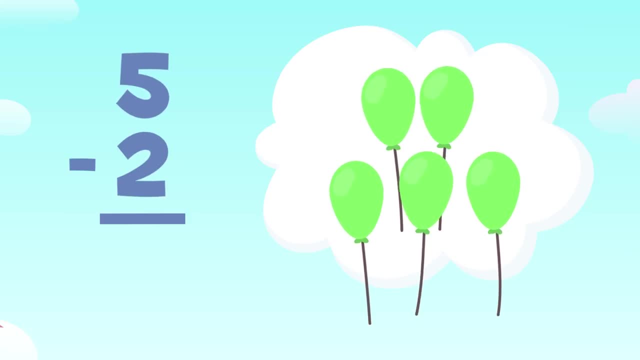 minus two. I'll aim at two out of five balloons. what will the result be? one and two- amazing, let's see how many we've got left. one, two and three: we've got three balloons left. the result of subtracting five from two is three. I love playing. 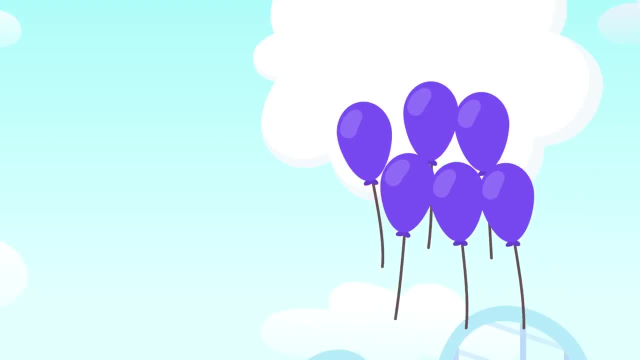 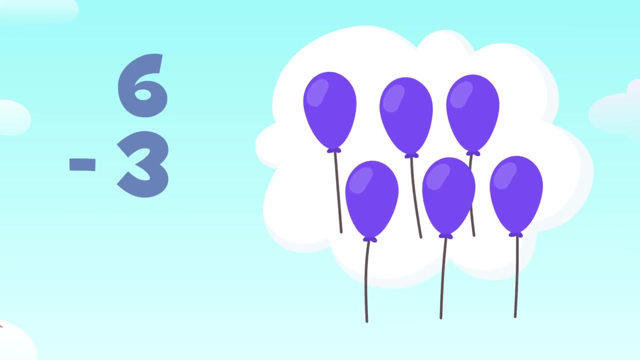 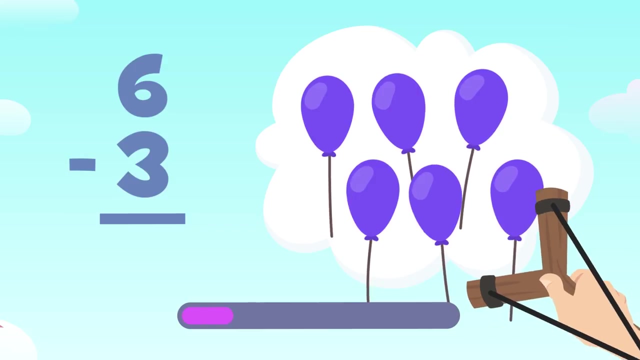 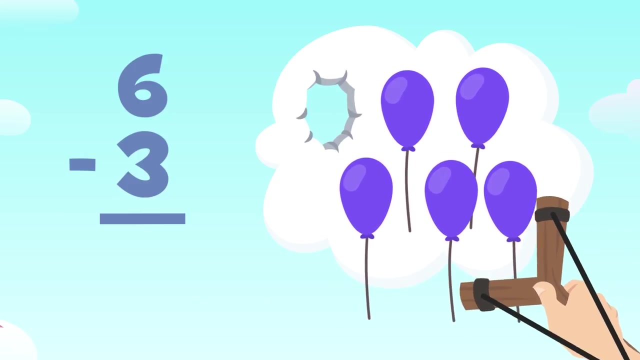 with my slingshot, you've let more balloons fly away. there are one, two, three, four, five and six balloons. how many will there be if I aim at three of them? the subtraction we need to do is six minus I'll aim at three. what will the result be? one, two and three- yes, let's see how many I've got left. one, two and three. there are three balloons left. six minus three equals three. doing subtractions is great fun. 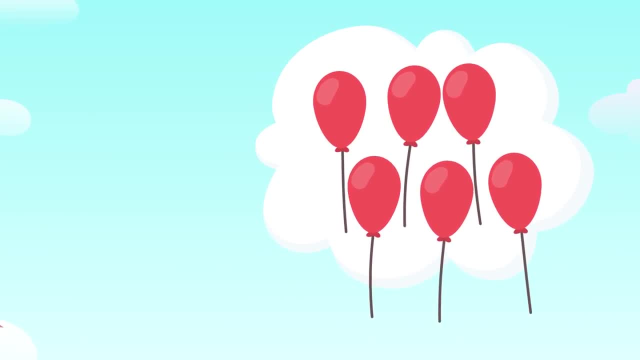 you've let more balloons fly away. there are one, two, three, four, five and six balloons. how many will there be if I aim at four of them? the subtraction we need to do is six minus four. out of six balloons, I'll aim at four. what will the 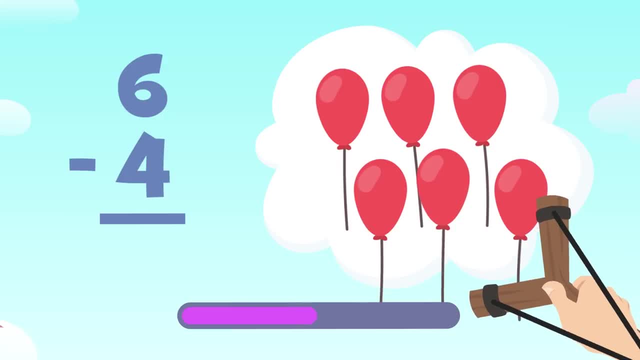 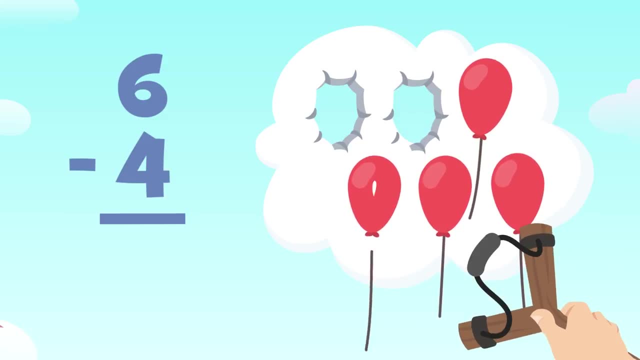 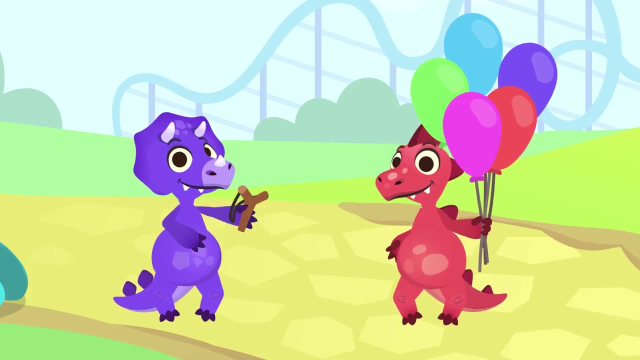 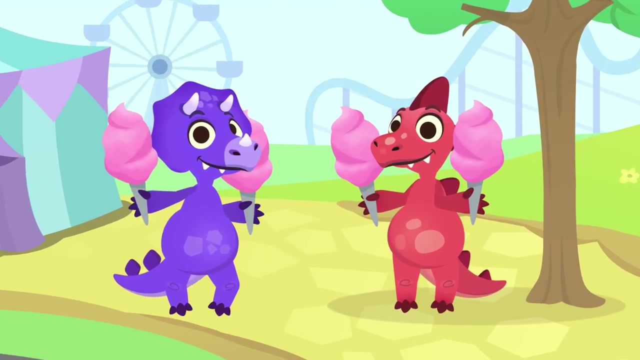 result be one, two, three and four. swell, let's see how many we've got left. we've got one and two balloons left. six minus four equals two. I love doing subtractions. you've run out of balloons, friends. well, at least you've learned how to do. 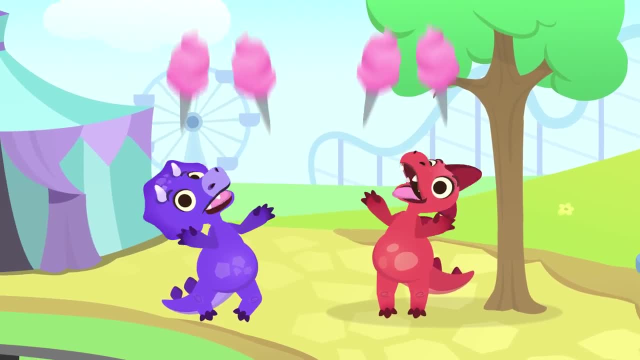 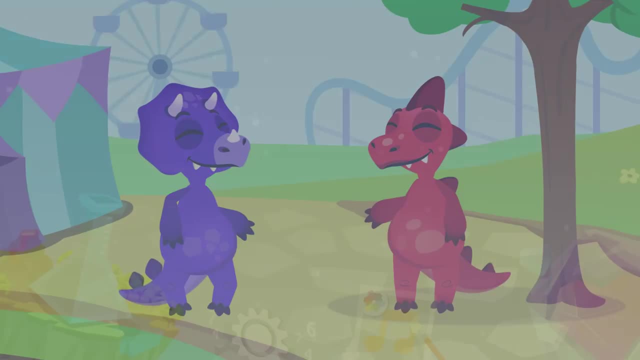 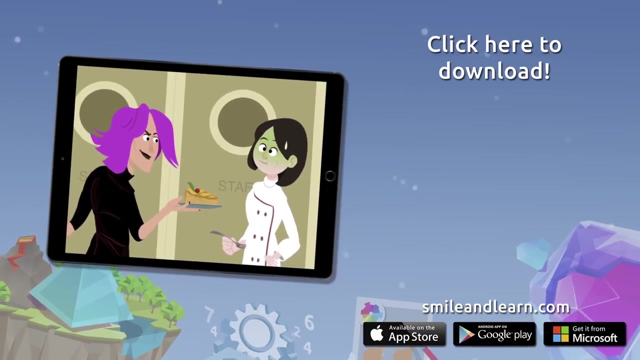 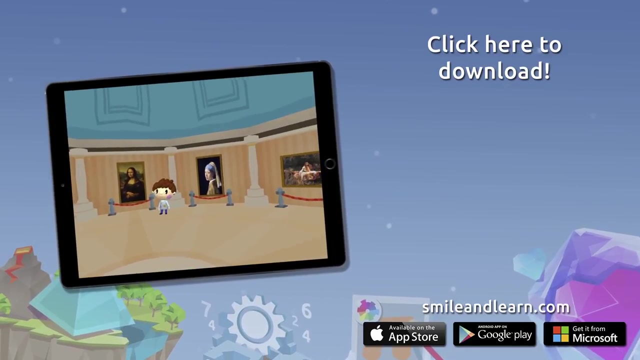 subtractions and you still have all that yummy cotton candy. do you want to keep on learning? try for free our smile and learn platform for a month and enjoy all of our games, videos and interactive stories. go for it. download smile and learn for free and learn on your mobile, tablet or PC.